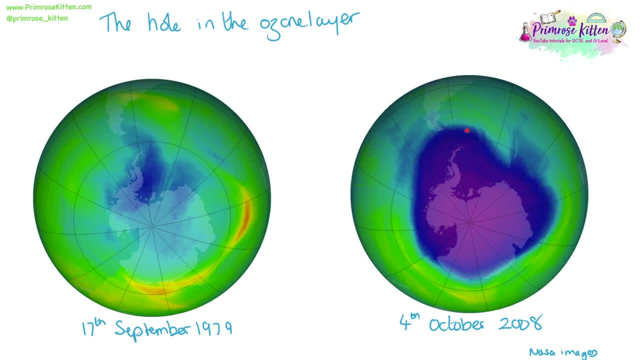 1979 and this is an image from 2008, and we can see that the hole is getting larger. From 1979 to 2008, there has been a massive increase. Now this is a problem because it means that that area, the life under that area, is not being protected from UVB. So if the ozone 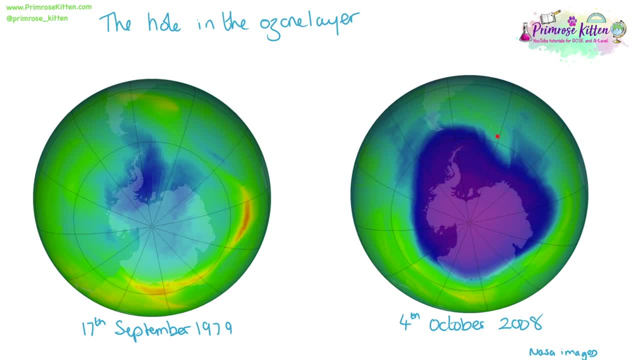 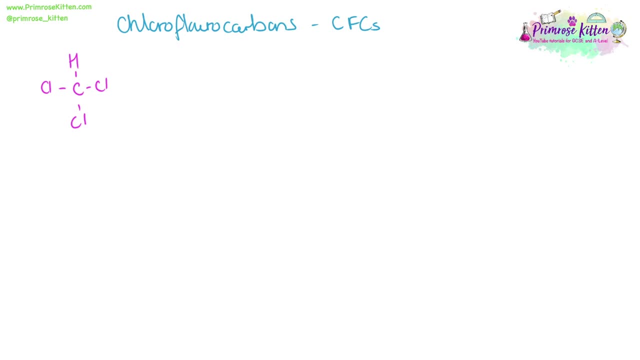 is not there, it cannot protect us. CFCs are chlorofluorocarbons And they are incredibly useful things. They can be used as solvents, as flame retardants or in refrigeration. They are very stable and this is due to the 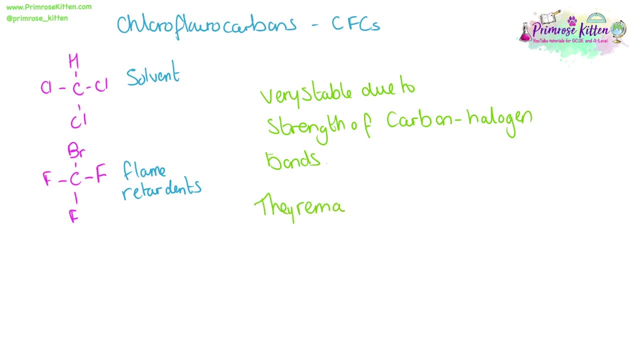 strength of the carbon halogen bond And they will remain stable, And they will remain stable, And they will remain stable Until they reach the upper atmosphere, and only then will they break down, Where they will form radicals, which are the problem. 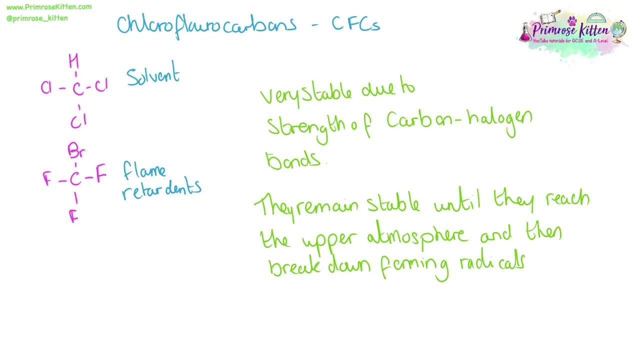 Now. CFCs were very popular for a very long time because of their properties. They are non-toxic, They are volatile, Which means they can easily be turned into a vapour, And they are non-flammable. CFCs are not toxic. 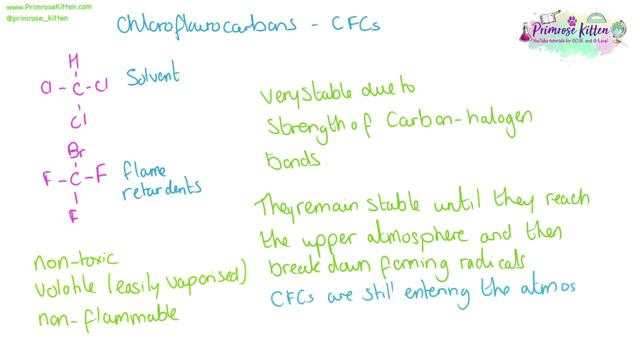 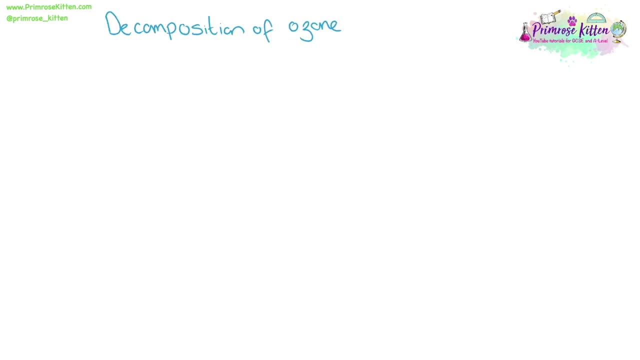 They are non-toxic. They are non-toxic. They are non-toxic. CFCs are still entering the atmosphere today, As they have a very long life. However, CFCs are responsible for the depletion of ozone. The UV in the upper atmosphere will break. 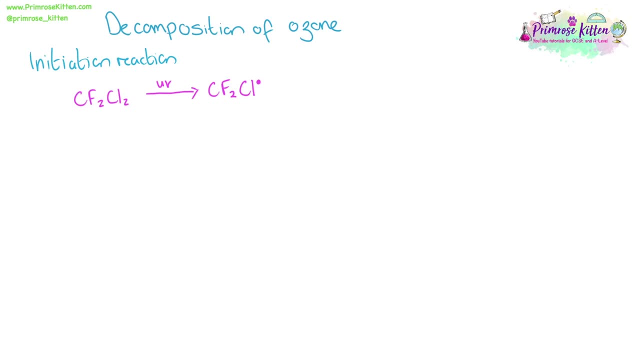 down that carbon halogen bond, giving us a halogen radical. These halogen radicals in the upper atmosphere will break down that carbon halogen bond, giving us a halogen radical. These halogen radicals can then react with ozone and oxygen further to create more radicals. 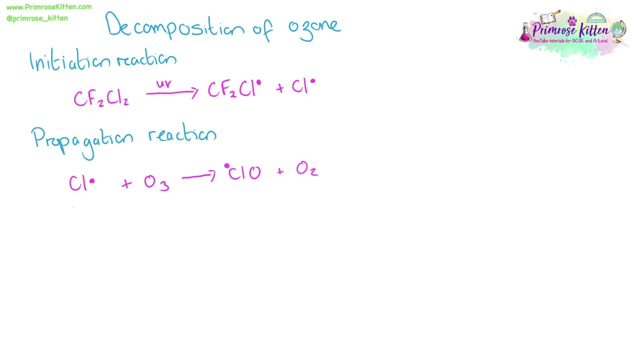 Chlorine radical will react with ozone to give oxygen And the chlorate radical produced in that reaction will react with oxygen atom to give the chlorine radical back again, making a propagation reaction and O2.. Chlorine radical. Chlorine radical, Chlorine radical.